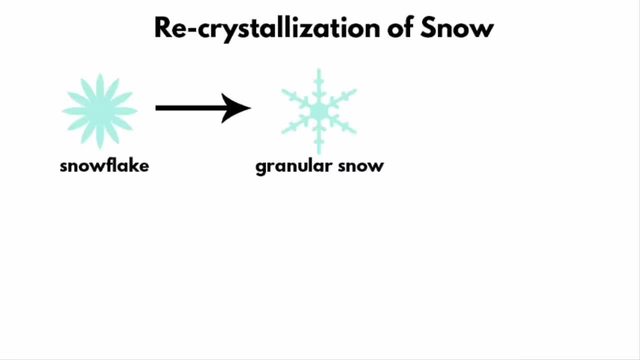 This compression forces the snow to recrystallize, meaning those tiny snowflakes becomes tightly packed together. As time passes, the density of these accumulated snow increases. If you go underneath a glacier, you will notice that the bottom layer of a glacier slowly 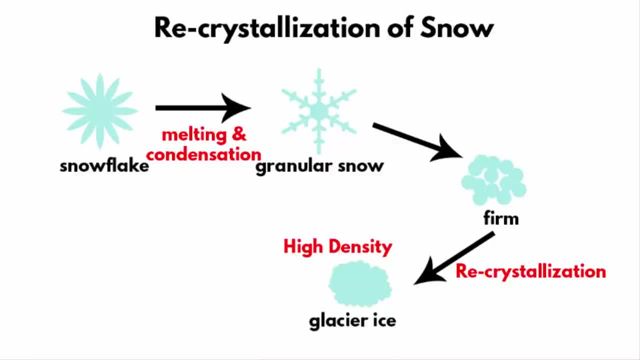 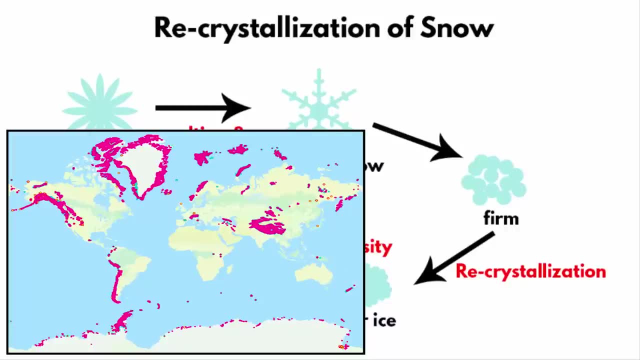 melts, Most of the water recrystallizes and forms like a rock. Here is a map that shows where in the world you will find glaciers. Mostly, glaciers occur in higher latitude and higher altitude regions. Glaciers are usually formed on steep slopes. I mean, that is the 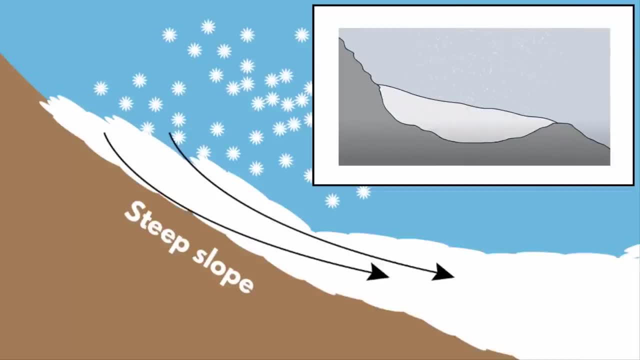 place of their accumulation. And if you look at the movement of glaciers- the bottom layer of the glacier, which is also called the glacier bed- it starts to melt And that literally reduces the friction between the glacier and the bedrock, making the entire glacier slowly. move. 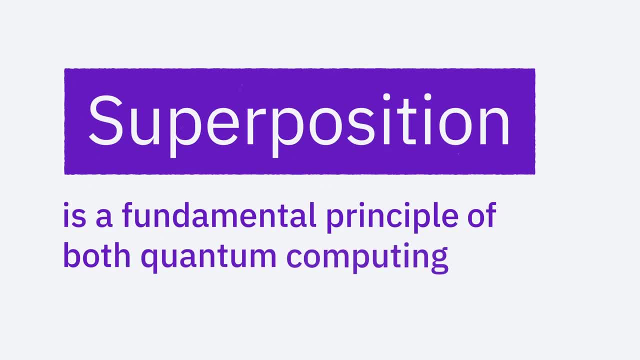 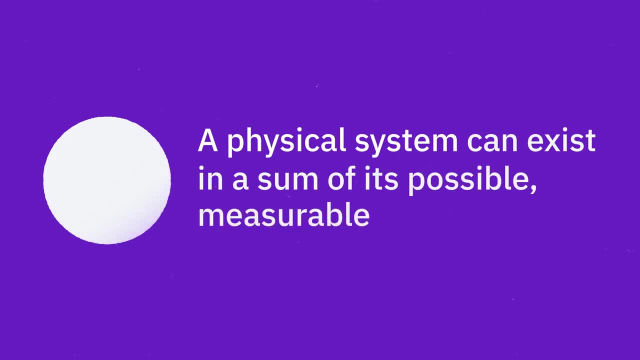 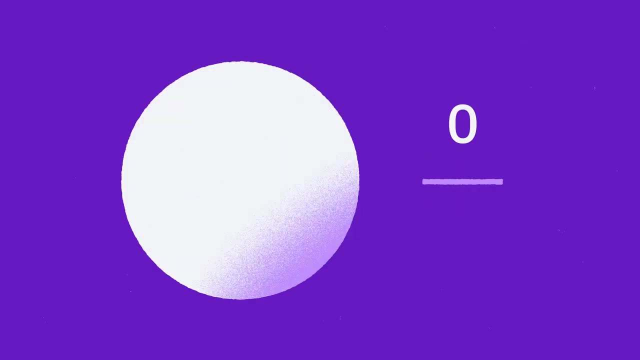 Superposition is a fundamental principle of both quantum computing and quantum mechanics. The principle of superposition states that a physical system can exist in a sum of its possible measurable outcomes. When talking about the superposition state of a quantum bit, the only possible measurement outcomes are 0 and 1.. 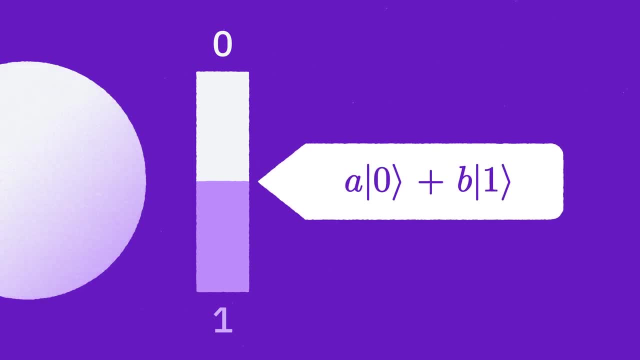 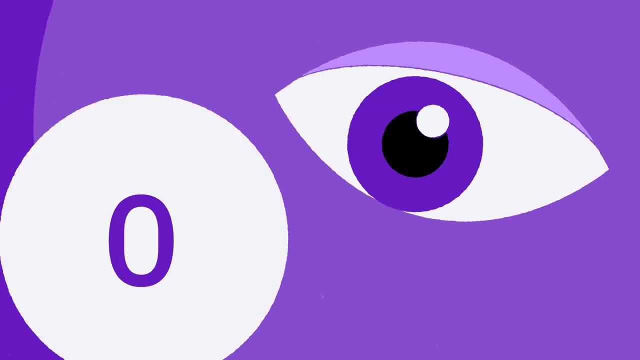 Writing this down mathematically would look like this: where the coefficient squared would represent the probability of measuring the qubit in either 0 or 1.. Once we physically measure the qubit, you will never find it in a superposition state. 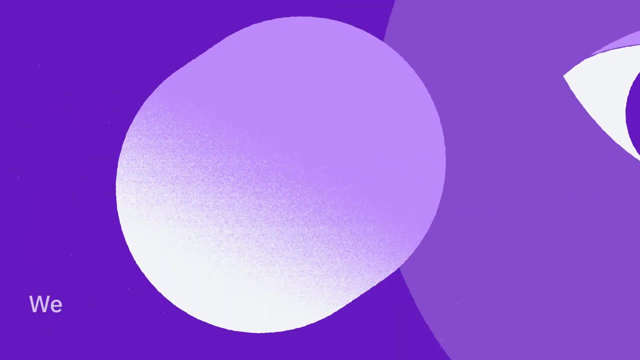 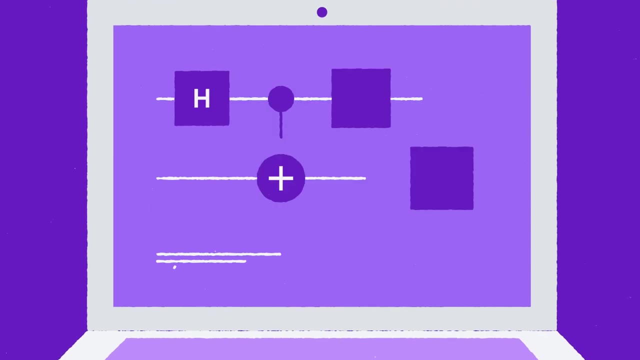 It will only ever be in the classical states 1 or 0.. We can never directly measure a superposition state- Quantum mechanics forbids this- But we can deduce it from the outcome of specific experiments. In Qiskit you can put a qubit into superposition by applying a Hadamard gate. 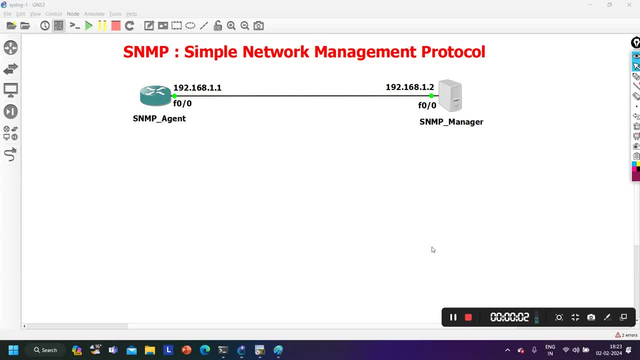 Hello everyone. once again, welcome to PM networking. Hope you all are doing great Guys. today, in this video we are going to understand SNMP protocol, simple network management protocol. So first we will discuss why we need SNMP protocol in real time. Then we will discuss.